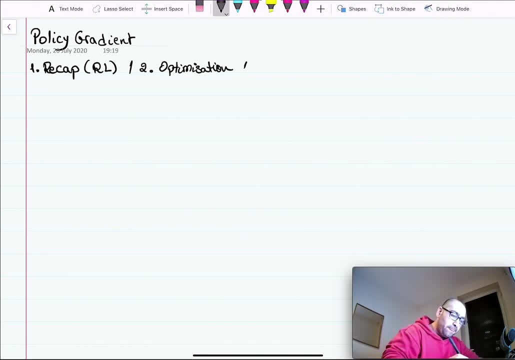 is in fact complicated or complex to solve. And then three suggest one of the algorithms to solve this problem, which is nothing but policy gradients. So let's start with number one and let's do a recap. So let's start with a recap. So you remember from maybe reading around or the previous lecture that we had a long time ago that a reinforcement learning problem is a problem that is interesting. 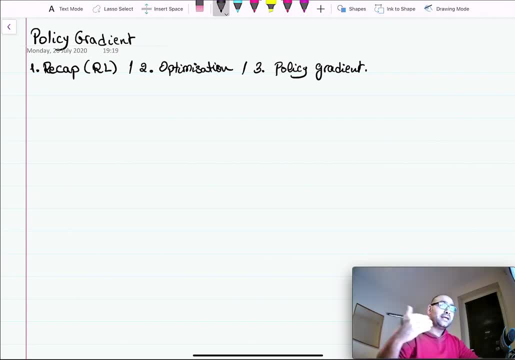 in solving sequential decision making under uncertainty. So our goal, really? so our goal is to operate in settings or learn in tasks which can be reflected or described as sequential, sequential decision making tasks under uncertain environments. So what that? what that actually means is that, OK, we have an agent and that agent needs to take a sequence right, Thus the word sequential here. It needs to take a sequence of actions in an environment that is typically uncertain. So we do not know this environment up front and we cannot precode all the possibilities of this environment up front in the lab. 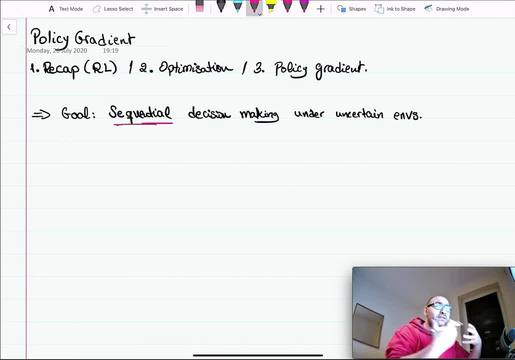 So what we need is we need to develop some system that is capable of dealing with this. Of course, examples of this are ubiquitous, right, Like if you think about robotics, or if you think about the AlphaGo game, or if you think about the chess, or or if you think about self driving cars, for example, or even logistics types of problems, then all these can be written as a special case of a reinforcement learning algorithm which is formalized, as we said earlier. 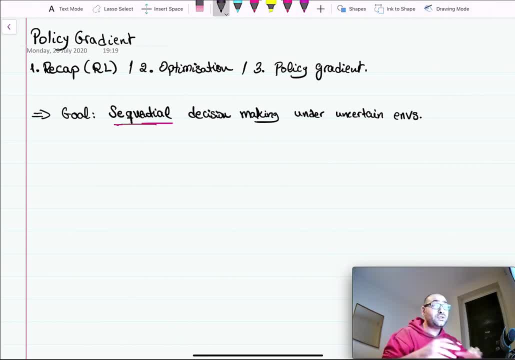 Last time using a Markov decision process, which is a way to formalize, to mathematically describe reinforcement learning problems, and that's Markov decision process, which we call then MDP. So MDP stands for Markov decision process. That was a tuple, So we're going to call that MDP. M Right And that is a tuple of X, U, P, R and a gamma. 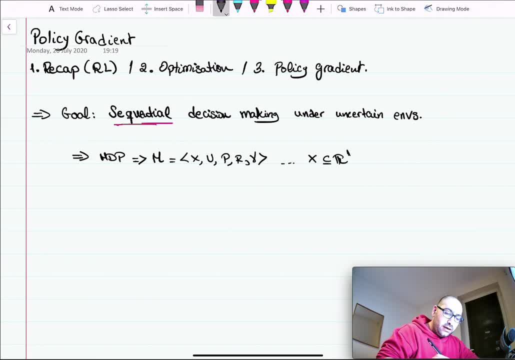 MDP is a subset of R, D and that simply means that X is a D dimensional vector, So it's a vector of D entries. Each entry is a real number and that describes the set of states. So where the car is in an X, Y plane, or or where the robot joint configurations are. And then U is another subset of R, M, So that is a action space, What actions the robot is allowed to take. 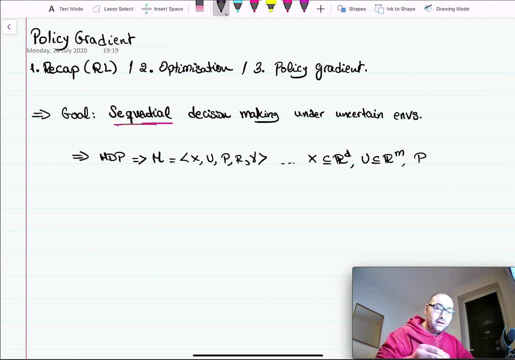 And then we also have the transition model P, and P is a probability density function. So that is a map from X cross, U cross, X to zero one And all that is saying. So what that is saying is that it's simply saying: OK, how will I be able to transition to a new state, given that I was at a current state and I applied a certain action? So how am I going to go to X T plus one, given that I was an X T and I applied a certain action? 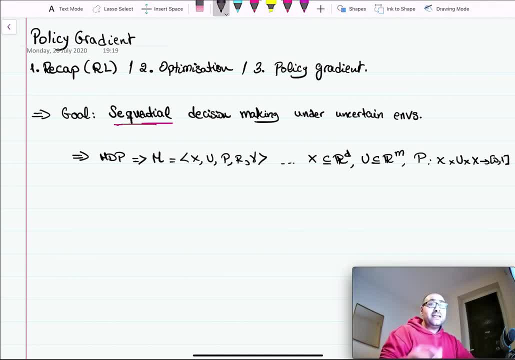 U T. Now the last ingredient I would need, or one of the last ingredients that I would need, is a reward function, R. So R is kind of a performance measure, So that tells me how well that transition I took was. So if I want to reach a goal, if I get closer to the goal, you know the distance minimizes, then you know I should get a positive number, Otherwise I'll get the negative number. So so R is a reward function, So that's a reward function. 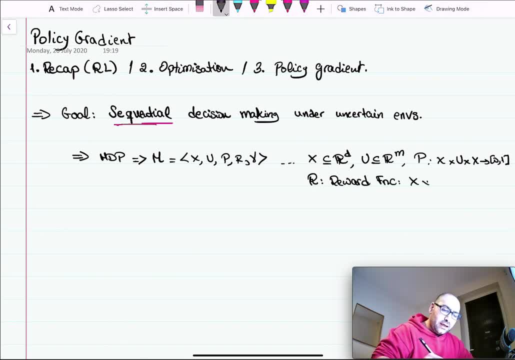 And it typically maps from states cross sections to the set of reels. So it's simply saying: OK, you were at a state X, T. you execute an action- a T, a, U, T, you'll get a number and that number is going to dictate how well or bad your transition was. 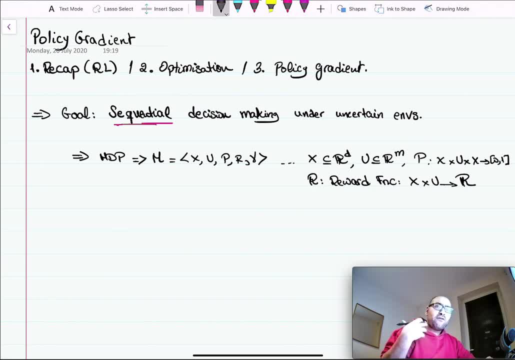 And, if you recall, back then we also introduced the notion of a policy and the policy was an action selection rule. So that was an action selection rule, Right, Action selection rule, And that action selection rule simply was a map. It mapped, or again, it was a probability density function, which is mapping from X cross U to zero one. 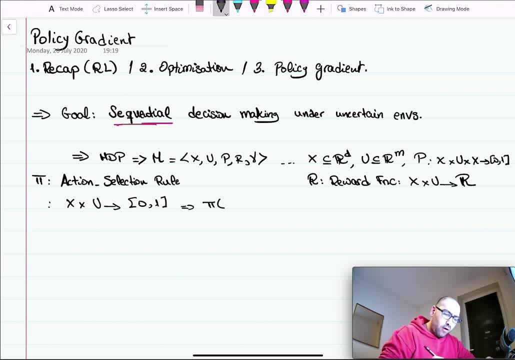 And now, when I say pi of U, given X, what I mean by that is the conditional density of sampling and action U, Given that I was in a state X. now, upon interactions with the environment, I end up computing or calculating a trace or a trajectory from that environment, which is simply a sequence of state action pairs. 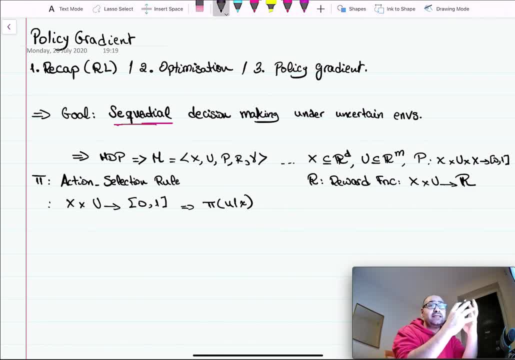 So I talk to this environment. I am at some state S or X, Sorry, in this case I apply an action U, Then, according to P, I transition to two X plus one, and then I get a reward for that, And then I. 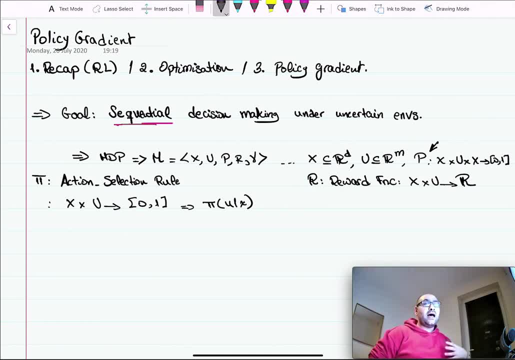 Repeat this process for some horizon T, And then I gather a trace, a trajectory, a trajectory which is this collection of state action pairs, And we call that trajectory back then tau, which was like X1, U1, X2, up to Xt. 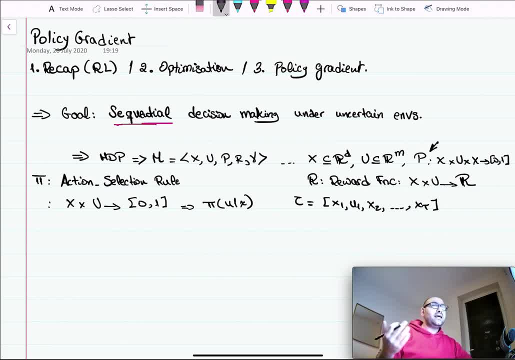 Now, by no means this is the only way of formalizing an MDP or reinforcement learning problem. I'm working with the episodic setting whereby I'm assuming a finite length of The horizon, But if you think about problems where you know you want to run forever, you can also formulate that. 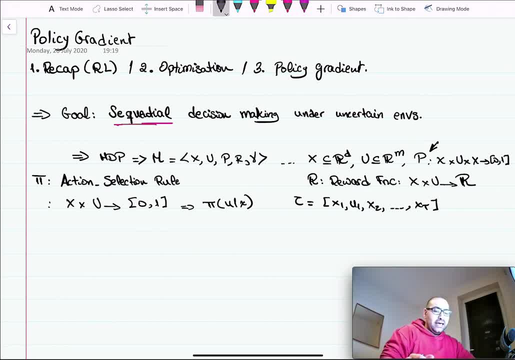 But as an infinite horizon type of problem. and also there is no need for the reinforcement learning algorithm to know either the reward function nor the transition model, and that actually differentiates it a little bit from optimal control, where optimal control tends to say: okay, look, I know something. 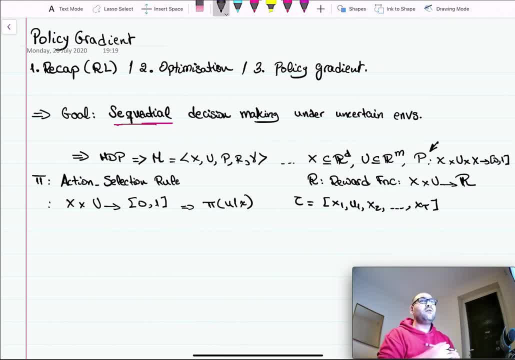 About these two. in our L model free- at least model free- settings. they just try to learn everything from scratch, right? They just try to learn everything by just interacting with the environment Itself. And now the goal, as we said last time, in reinforcement learning, is to try to find some sort of a policy, right? 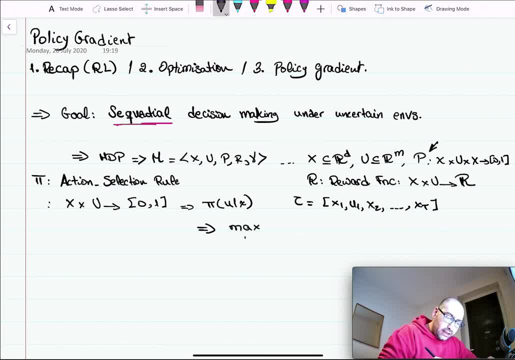 So we want to find a policy pie that maximizes. So we want to find a maximum right Over, Over Over the expected total rewards. So Tao is sampled from P pie of Tao And now we have a reward of Tao. 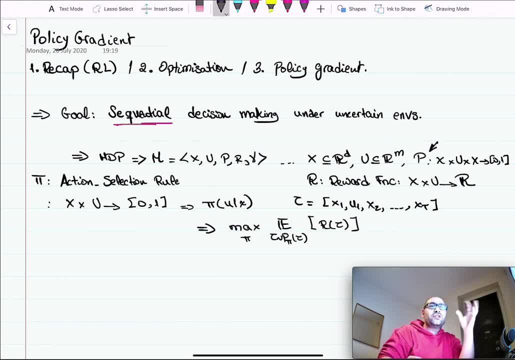 So now, before going into the mathematical understanding of this problem, it is also very intuitive to see what this problem is trying to do. So are of Tao, right? So this, this, this, this part here are of Tao. That is the total reward. 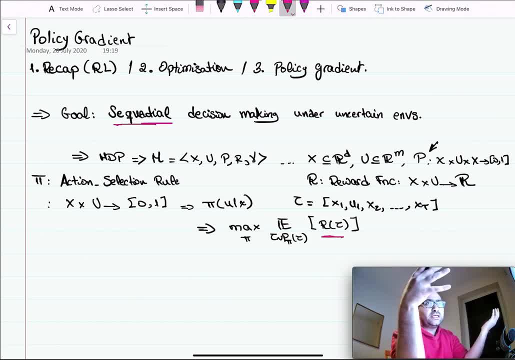 You would get you know, across a trajectory, across a trace. So for every transition you made, you know, going from X2, applying U2 to X3. What has happened is you got the reward value. Let's say we sum them up, over and over this horizon, T, and that will give me R of Tao, R of the whole trajectory. 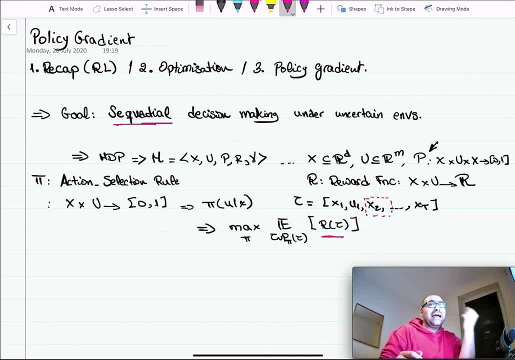 Well, my goal is is: I want to find such an optimal action selection policy, a policy pie, So a some distribution Of U given X, such that on expectation or on average, all right, over all these possible traces, my expected reward is maximized. 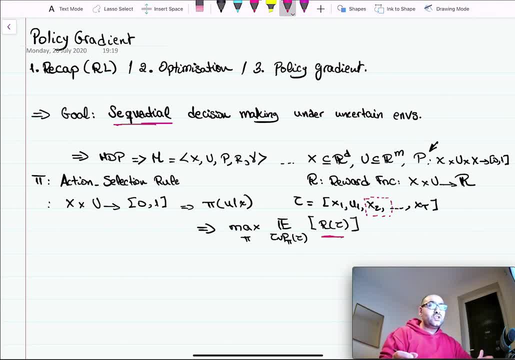 That's, that's kind of what I'm looking for, right? So so all I'm trying to say is: okay, give me that policy pie that, in expectation, you know, will have its maximum total rewards, And back then we also back then. 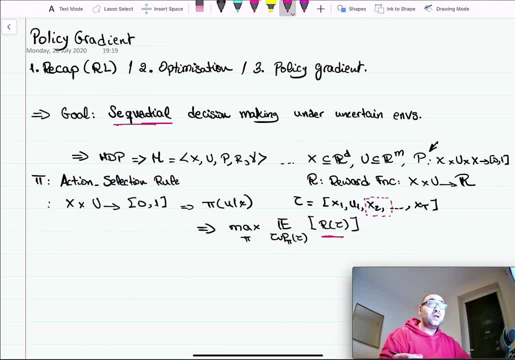 We also Talked about what P pie Tao was and we said that this P pie Tao- right, It actually can be factored using the chain rule of probability and the Markov property into something that says it's a P of X1, which is kind of the initial state distribution times, the product over time. 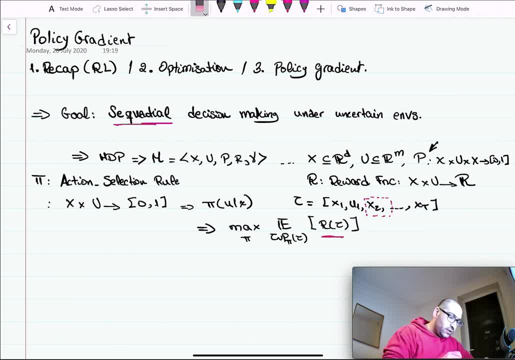 You know what? Sorry, let me, let me, let me get more space here. So so we said last time That P pie of Tao Is going to be written as some initial state distribution times the product over time, right? 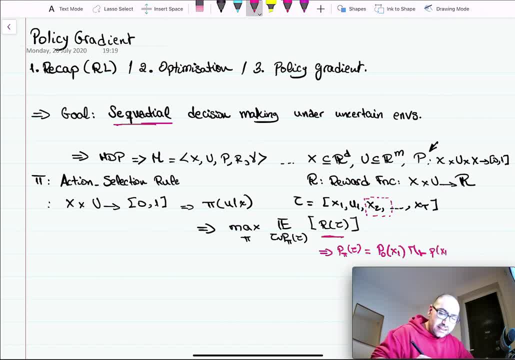 Comes the product over the time steps of P of XT, plus one which is my transition XT, UT right times the policy pie of UT given XT. So so now we kind of Understand what the reinforcement learning problem looks like, And it is a problem which is defined as an MDP, and that MDP is made of a state, space action, space transition model, reward function and a discount factor. 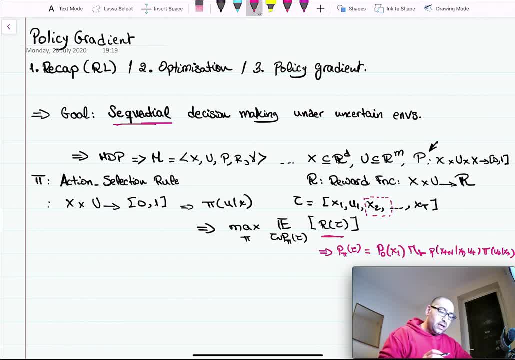 And then we also said, okay, in an MDP, the goal is to find a policy pie, which is an action selection rule that actually tries to solve this problem. So I believe that's where we have ended last time right, But we have not. we have not had the chance to speak about solution methods and what solution methods look like for reinforcement learning. 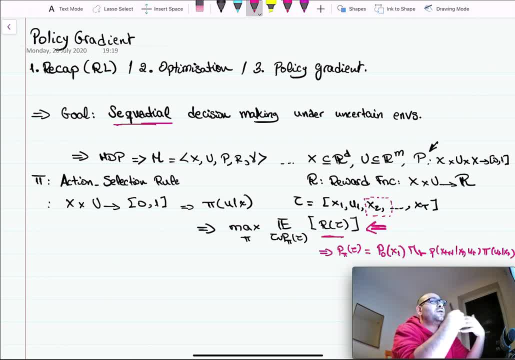 Now, of course, there are tons of literature and this on this, and then you can read a lot about it. I'll just give you some survey, a little bit of a survey, about what methods exist in order to solve reinforcement learning. methods or reinforcement learning. 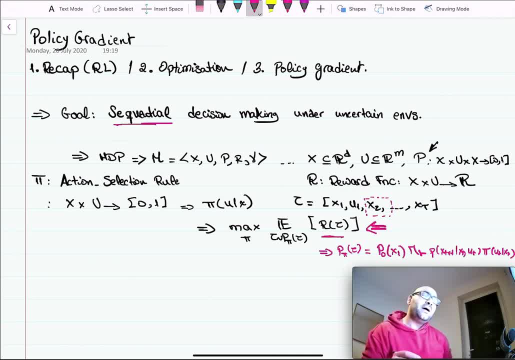 Problems, Sorry, and also we will. we will talk a bit about policy gradients in a bit more depth and then, hopefully, in later lectures, We built on top of that. All right, so we know all this stuff. So now let's, let's try to go forward. 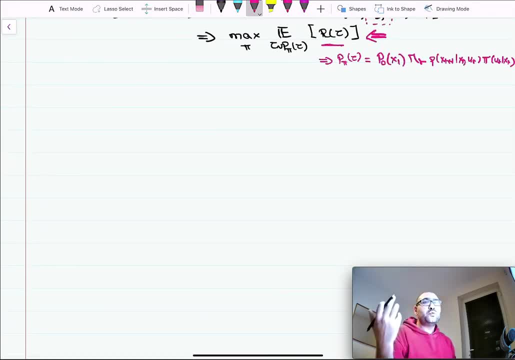 Right. So this is our problem definition. We understand it, We know what it means, but now how do we solve it? So it turns out that there are maybe two big directions in the way you would. you would try to To tackle reinforcement learning methods. 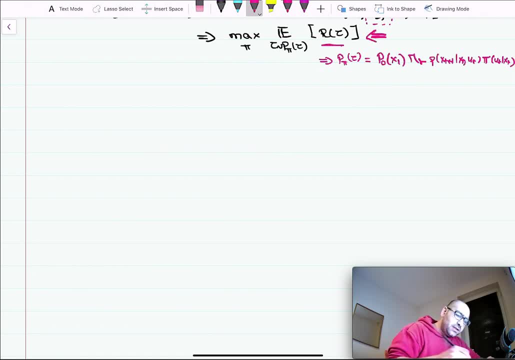 So solution methods to this problem. Let's call this problem P1.. So let's call this problem P1.. All right, So solution methods to problem P1. right, can actually be split in two, So they can be split into what we call model-free algorithms. 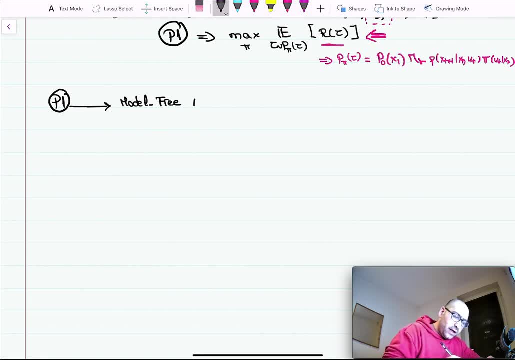 So these are one type of solution methods- model-free algorithms- And the other type of methods is what is called model-based algorithms. So the other type is called model model-based, right? So? so it is a model Based algorithms. So all right. what is the difference between these two types of algorithms? 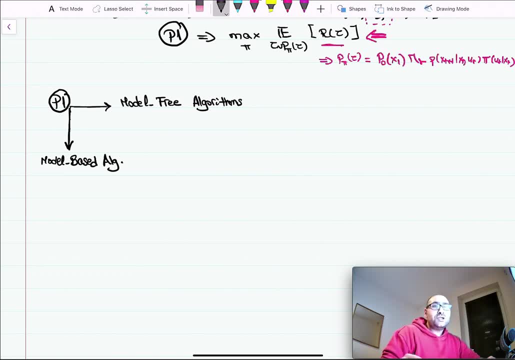 Well, model-free algorithms. They just try To learn by directly talking to the environment, right So? so the architecture of the system is pretty simple. It's like an agent and environment. They talk to each other. the agent takes actions and then it gets some new states and rewards, and then it collects these trajectories. 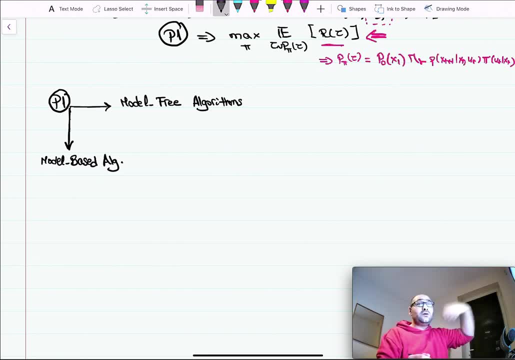 We talked about tau above, and now our goal is, you know, to try to, you know, solve this problem, and, and the way we will do it is by just doing that. We will not learn anything on top. Now, This is interesting and it has been widely applied in reinforcement learning, and I'm sure you heard a lot of these types of algorithms. 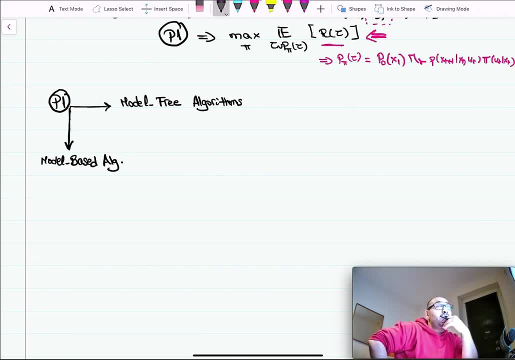 For example, dqn is one type of these algorithms. you know a3c, DDPG, you know all this stuff are kind of model-free algorithms. but now on the model-based side, The the idea, Oh so so before going to the model-based side, we realize that model-free algorithms though, 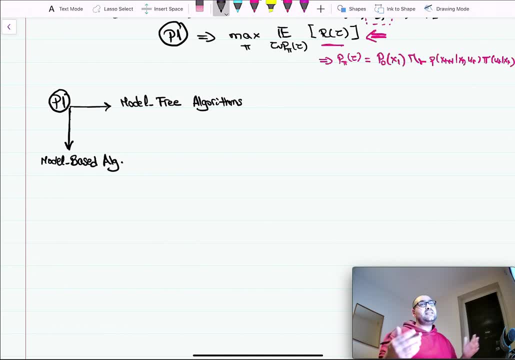 They have been successful. They're very simple and efficient. So what is sample inefficiency? It means that the amount of times you interact with the environment is really large. So if you look at any of the nice works by by colleagues on reinforcement learning, you realize that if you look at the x-axis, which is like the number of frames you need to learn, you will get numbers in the millions. 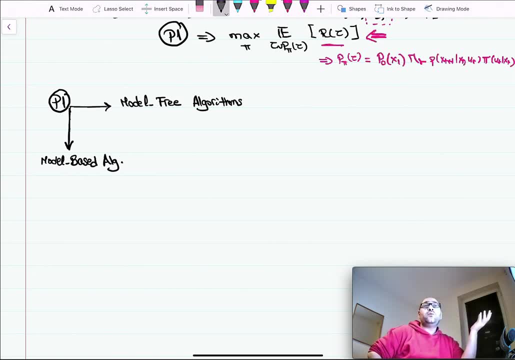 And now numbers in the millions are actually not that useful for real-world applications. They might be really really cool for, like a computer game, But they're not. They're nowhere near, you know, being applied to to the real world, model-free, a model-based algorithms. 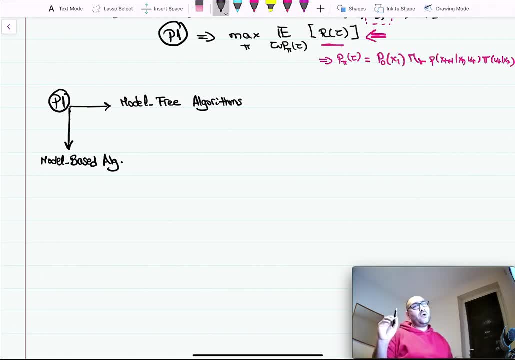 On the other hand, they work in a slightly different way. So they say, okay, I'm going to get this data from the you know, from the environment. rather than just basing my knowledge on this data, I'm going to build a model of the dynamics and, potentially, the reward function, and then I'm going to try to learn through using that. 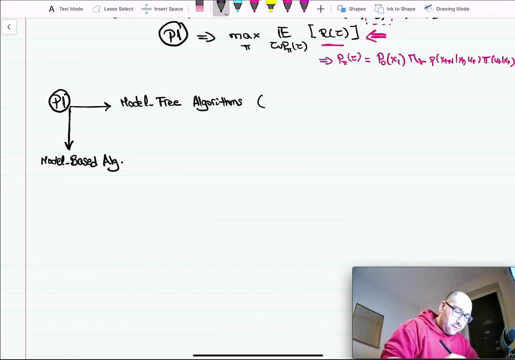 Right So so model-free algorithms like kind of like learn directly and the model Based algorithms They build a surrogate MDP or surrogate model and then they learn in that model. Now, model-based algorithms are really cool because they're very sample efficient. 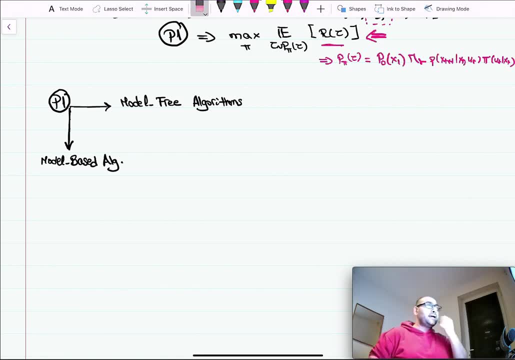 And one of the most famous ones is Pilko, that I personally like a lot and- and I think it's- it's one of the best algorithms that has been created for solving reinforcement learning. and a word or two on some new benchmarking papers popping up on this. 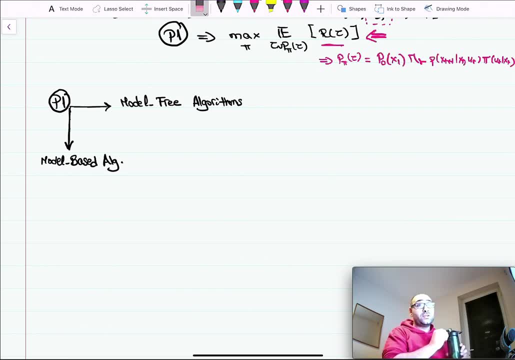 I'm not sure, like we have never gotten Pilko results that they report, So I'm not sure how they got these results. However, model-based algorithms don't successful. They still cannot generalize really really well to high dimensions. If you look at the new papers from Google called dream to control, 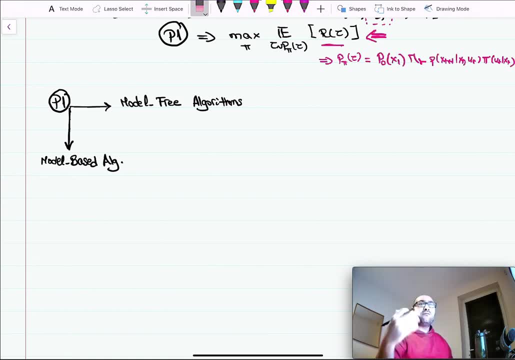 That's actually one method that is kind of getting there, But the numbers are still kind of e to the power 6.. Now, in general right RL algorithms can be further split into like direct versus indirect methods And indirect methods. they build kind of a indirect quantifier of the policy, such as Q functions, while direct method 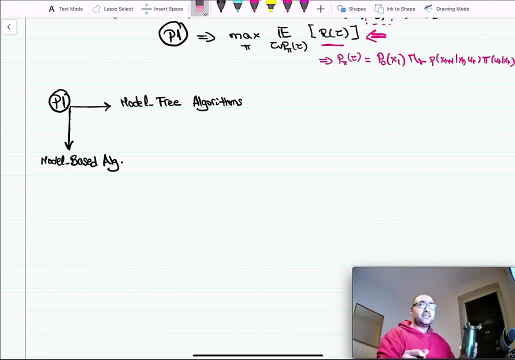 They just parameterize the policy and they just try to operate in that space. So we will hopefully get into discussing all these as we go, But what this lecture is going to be about is direct methods. So what direct methods are going to do? 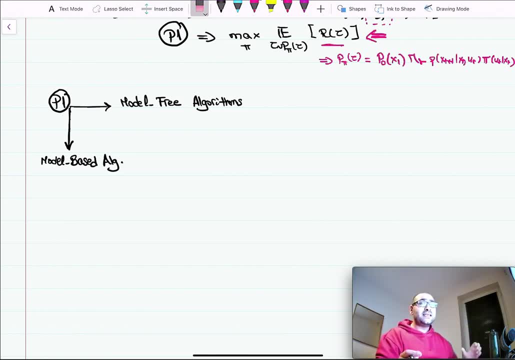 It's going to parameterize the policy pi by theta. So it's going to say: okay, What I'm going to do now is I'm going to introduce some neural network, Let's say, that has some theta, unknown parameters, theta, and that parameterizes the policy. 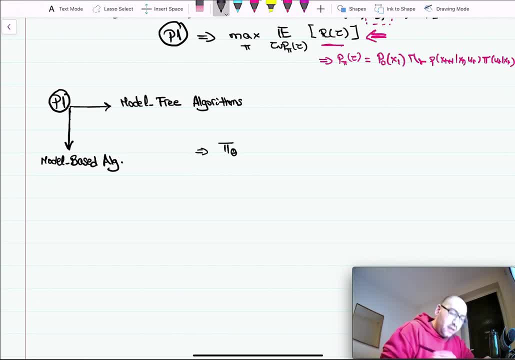 So now I'm going to, instead of writing pi, I'm going to write pi: theta All right of UT, given XT And what that looks like. You know. you can think about it as like you know, like the way you like, whatever model you would love, whatever model you would like. 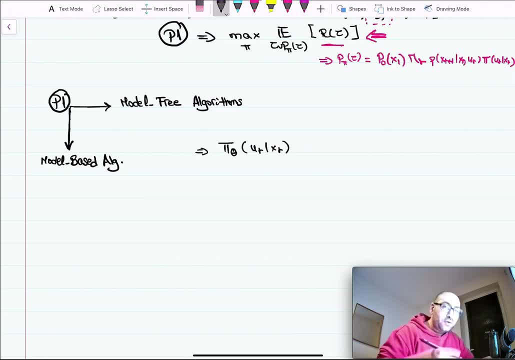 You just can use as your policy. So, for example, you can use a deep network. you know where you okay, on the input layer here You would put an XT, which is kind of your state, and then you know you have like a network here with some some connected units, right. 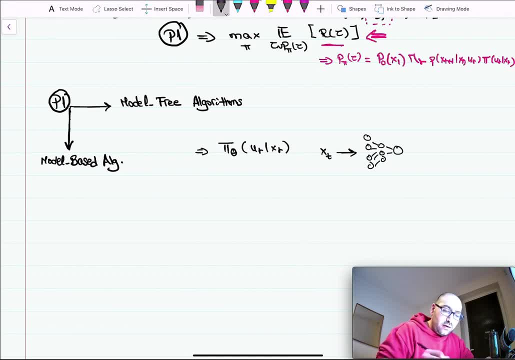 So this is like a fully connected whatever, and then here you will have your output action, UT. All right, Now, of course, this pie is a distribution, So you should output the distribution from your neural network, And the easy way to do that is you just parameterize a mean and a covariance of, like a Gaussian distribution, for example. 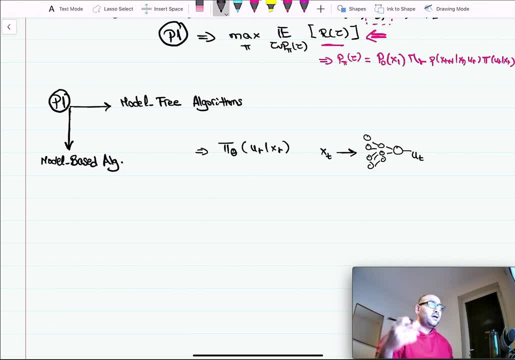 And of course there are much more interesting types of. there are much more interesting types of parameterizations that give you densities already, But maybe the most commonly used one is this: network is outputting like a Gaussian Mean and covariance, which is really equivalent to just adding some noise to this output: UT. 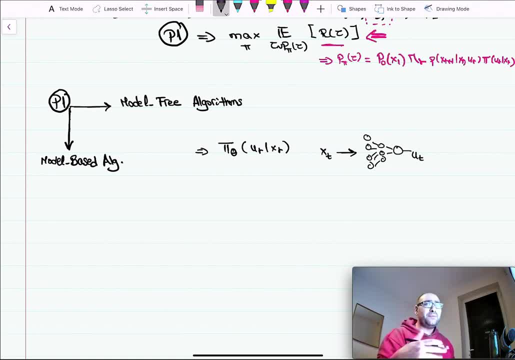 But anyways, it does not really matter much. The idea is that you know you just can parameterize it whatever you would like, you know, in whatever, in whatever form you'd be really interested in. So now, with this, we can transform problem one into problem two, and problem two is simply going to be okay, rather than looking for the space over some probability distributions, which is extremely. 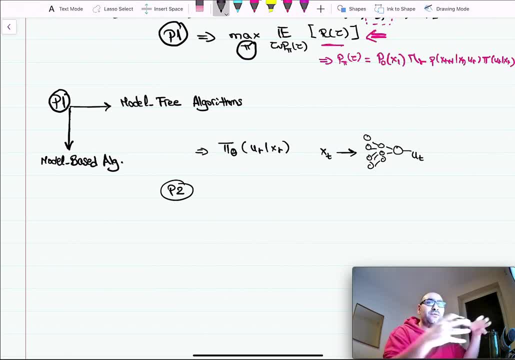 Hard to to understand and deal with. we have effectively restricted that space into a parametric form by enabling, by, by introducing this theta. So now looking for different theta will give you different distributions, but these distributions are not infinite possibilities. They are restricted within the hypothesis space enabled by theta. 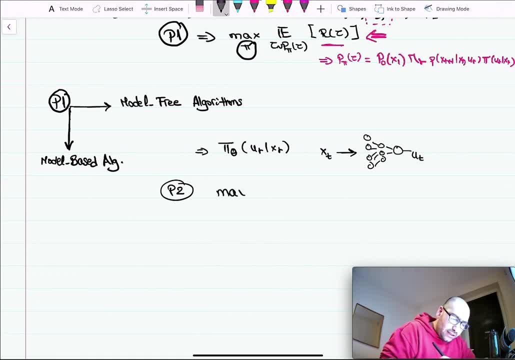 So now, what you can do is now you can say, okay, instead of doing that, I'm going to know, maximize over theta, All right. And now, instead of doing e over Tau pi, it's going to be e over Tau sampled from P. theta of Tau. 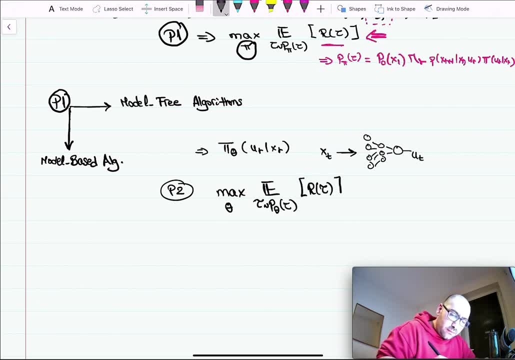 R of Tau, Right. So all I've done to go from here to here, So all I've done to go between these two is I just introduced, So these two here, So going from there to there, I introduced this parametric distribution by theta. 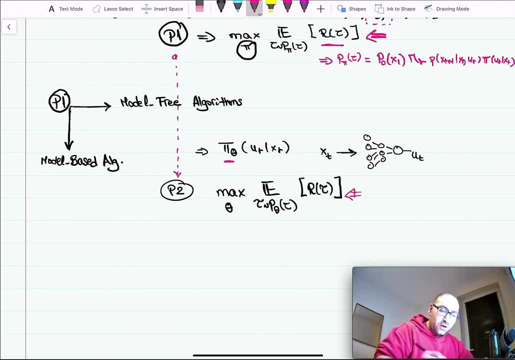 And now that's my problem that I Would like to solve. All right, So how would you go around solving this problem? Well, I mean, at the end, you know, if we think about it, this is just a standard optimization problem, but it's kind of stochastic and a bit messy. 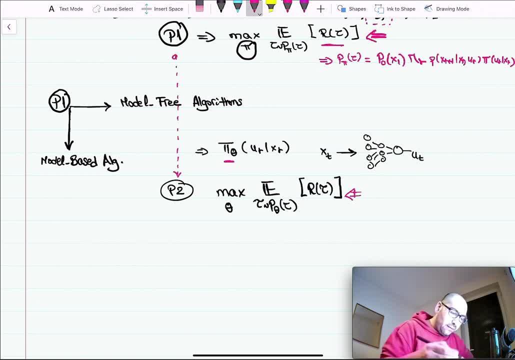 But, but it's still like it can be seen as okay. I'm going to try to maximize some function of theta, right, Some function of theta where, where that function is, you know whatever is written here. So okay, So let's call that J. 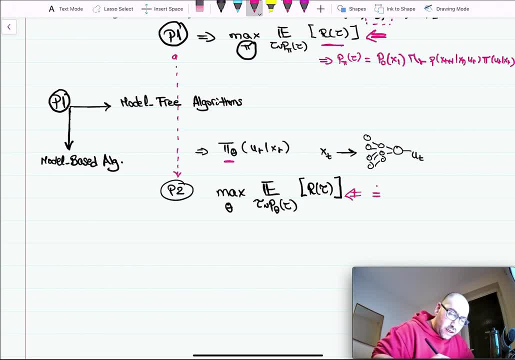 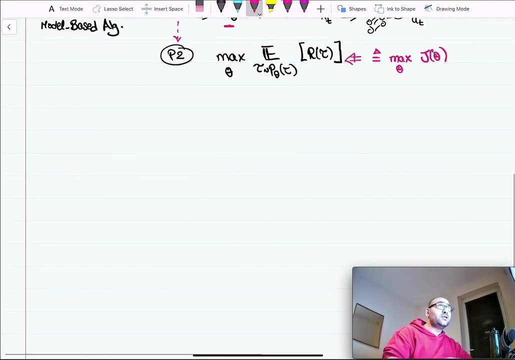 So, Essentially, what we're going to do is we're going to say, okay, I'm going to maximize with respect to theta, J of theta, where J of theta is just this expectation: Tau, R of Tau. All right, Good. So that's kind of now our optimization problem that we would like to tackle. 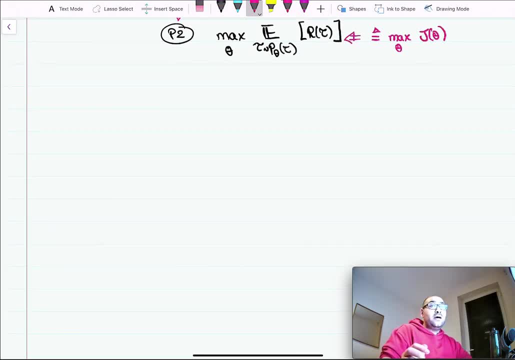 All right Now. Now please remember the definition of the expectation. So so, because if this will become interesting later, so remember that we can write the expectation as Kind of the integral right, So it is the integral over P theta of Tau R of Tau right. 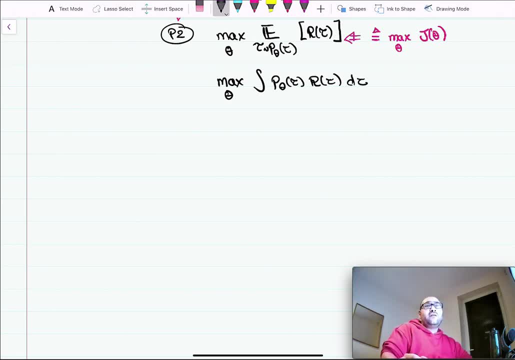 D, Tau. So that's kind of the definition of the expectation. It is the integral over the density times the function. I'm interested in detail Now. you might have seen this, maybe in a discrete setting where you have summed PIXI. This is kind of an continuous analog to that where rather than summing we just integrate. 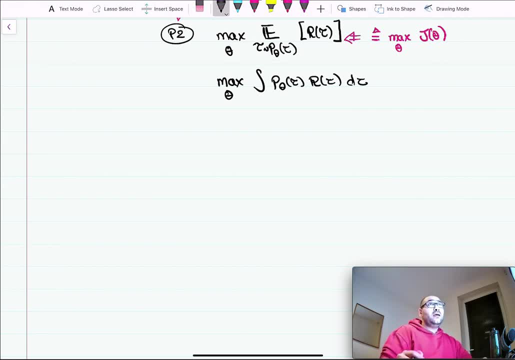 All right, great, So. so that's what we have and that's our J of theta, So so. so, that's our J of theta, All right. So how would one, you know, go around optimizing this? As I said, this is just a standard, you know, like a standard optimization problem. 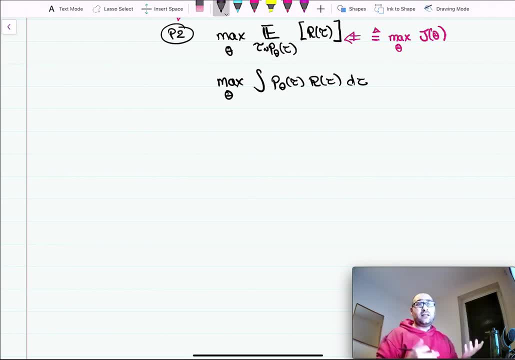 Let's try to do gradient ascent type of method right now. Why ascent, not descent? Because this is a maximization. So rather than the negative sign, you just have a plus sign. All right, So if I'm going to do gradient ascent, 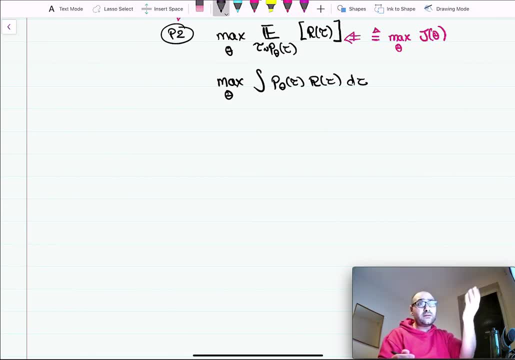 Or something like that. then I'm really interested in computing the gradient right of this J of theta. So so I'm really interested in finding the gradient Of J of theta Right now. that is, the gradient with respect to theta of J. 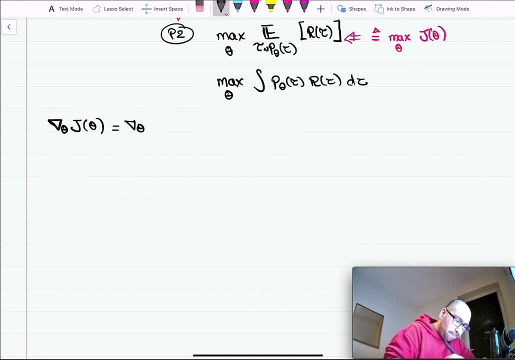 Oh sorry, of this integral Of P theta Tau R of town, T, town, Right, So so now. so now, the gradient of J is just the gradient of this loss function, which is nothing but this expectation thing. Okay, Now we have a mess because, first of all, we have two questions to do. 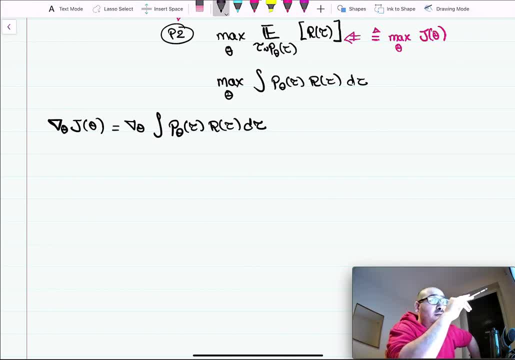 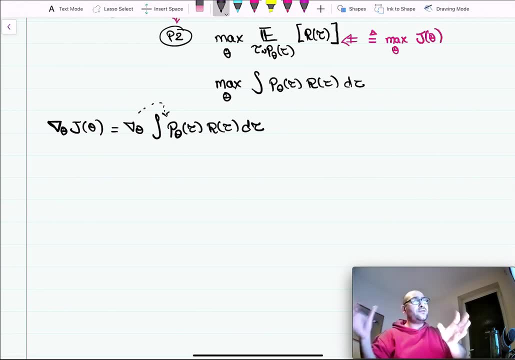 The first one is okay. or to answer: Can we get the gradient under the integral? Like, can I? can I get the gradient in there? All right. And now it turns out that under some further theoretical considerations, We can actually put the gradient under the integral. 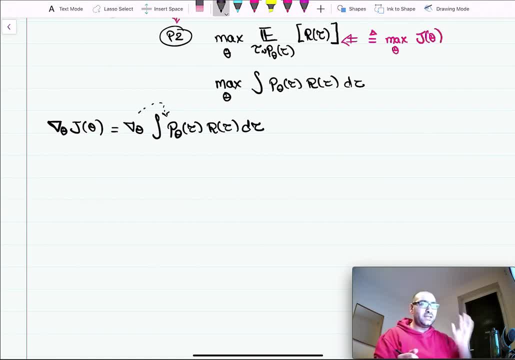 So we can put the gradient under the integral, So we can put the gradient under the integral, So we can put the gradient under the integral, And specifically, because the limits of this integral is kind of independent of theta, So you can, you can put things in and then what will happen is is you can, you can now rewrite this as the gradient of theta, of P, theta of Tau, R, of Tau. 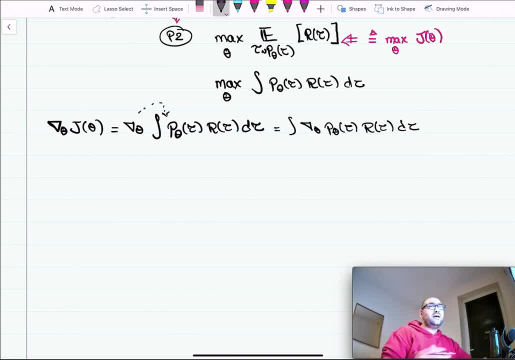 The town. So all I've done from this step to this step is just putting the gradient, you know, under This integral. All right, fantastic. But now we still need to compute the gradient of some very messy probability density function of a trajectory. 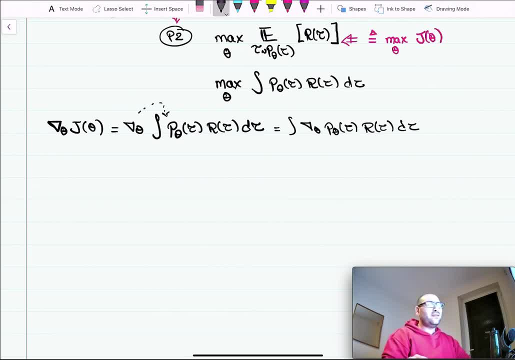 Right, Okay, So to do that. I think it's called the Fisher identity. People call it likelihood ratio method, but it has different names in different fields, But it's essentially one similar trick. The trick says the following: when I'm going to compute the gradient of some function of a, 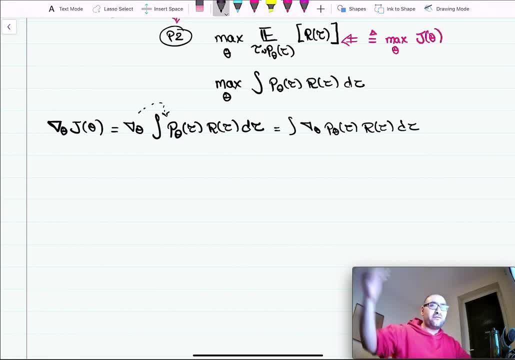 I'm going to try to compute the gradient of log of f of x. So let's see why that is the case. So do you remember the logarithmic function? So so imagine you have log of f of x And now imagine you take, you know the the gradient of this. 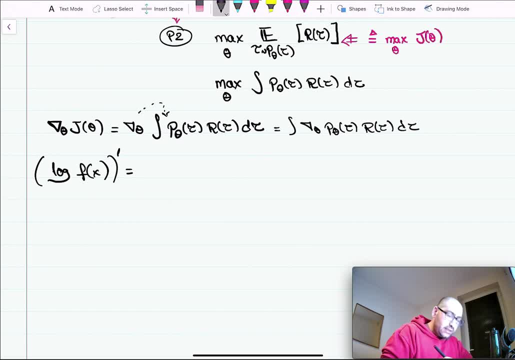 Yeah, So what would that gradient look like? So, so that or that derivative. in this case is just a 1D example for now You will get nothing but f prime of x right Over f of x. Yes, So now that means that if I cross multiply right, I would say that f prime of x is nothing but f of x. 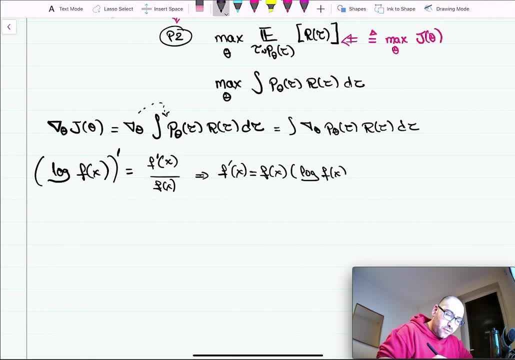 Times, the log of f of x prime. Right Now you might say: why? why are we doing this now? You will see in a second that this will transform this gradient of an expectation on its own, But even also, like, maybe just intuitively. 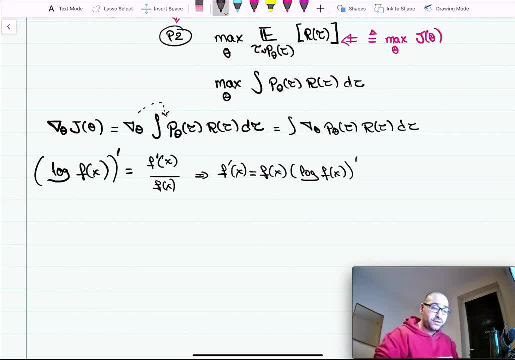 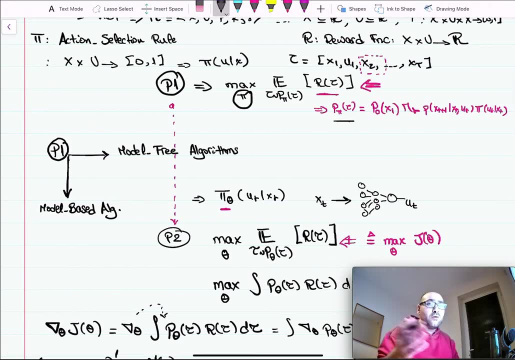 Remember that this p? theta of tau had this product over time, right? Because this p? theta of tau is nothing but this, right? So now it had this product. Now it's interesting because the log would make it a sum, So it's kind of easier to compute the derivative of a sum rather than a derivative of the product. 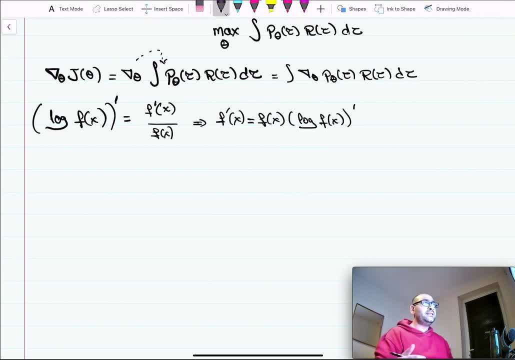 And, by the way, you can prove a similar identity for high dimensional cases. So, instead of taking a derivative, you take the gradient. That's also fine, You can do that, But now what we're going to do is is This: allows me, if you look at this right. 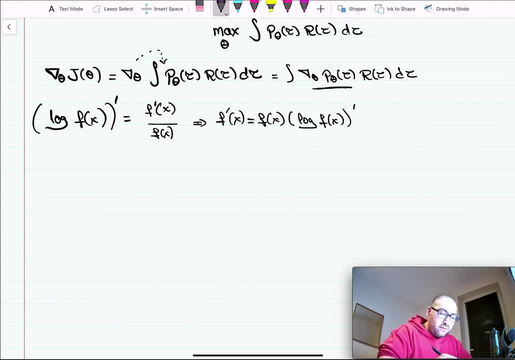 To rewrite the gradient of this p of theta of tau right In a form which has this log gradient in it, right? So? so this allows me to say: I mean f, prime is like the gradient, right, So you can say okay. 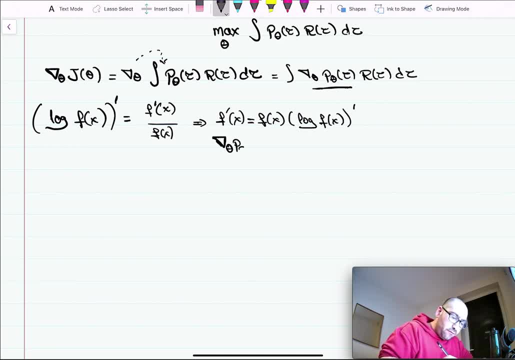 Now this is the gradient with respect to theta of p. theta of tau is equal to remember our f. in this case, If f, prime is gradient, then f is the, not gradient, Which is p, So now. so now you get p. theta of tau here times the gradient because it's the derivative of log of p. theta of tau. 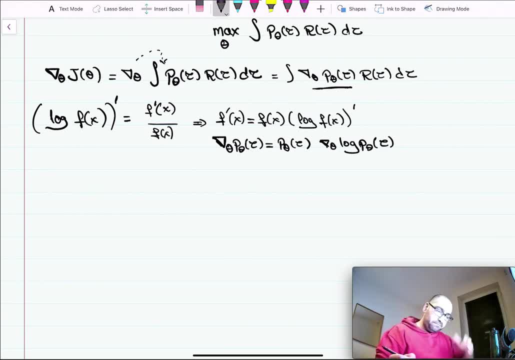 Now this trick, as I told you, it has different names, So we call it likelihood ratio, Some people call it reinforce, other people called Fisher's identity. Yeah, but anyways, now I can take this result which I got here Applying this log the trick, right. 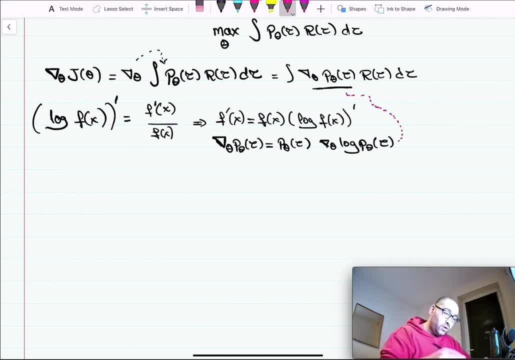 And just try to stick it there, right? So what will I get? Well, okay, I will get. if I just put it there, I will get the integral of p, theta of tau, right? I'm just substituting this back in that equation. 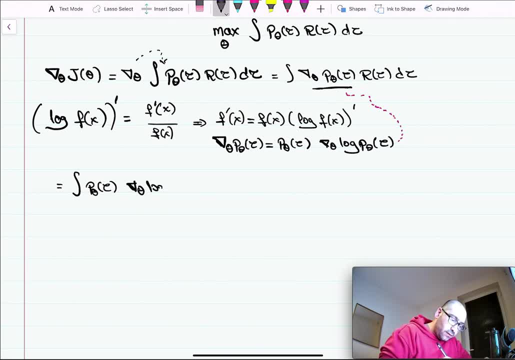 Then you would going to have a gradient theta of log of p, theta of tau, right? So so I just, yeah, substituting it Up times the reward r of tau d tau. Now, this is actually pretty cool for two reasons, right. 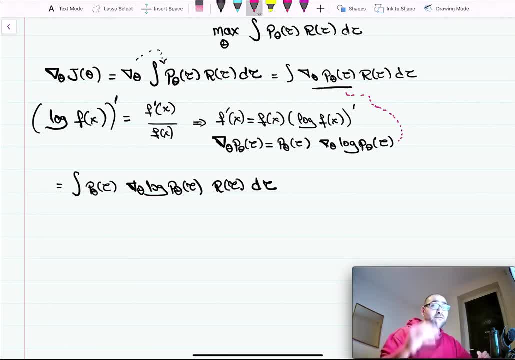 So the result we got- because- remember, the definition of an expectation right- Is nothing but the integral of p, the density times, whatever the function is- You can clearly see from this equation that you have an integral of p. So you have that part here, right? 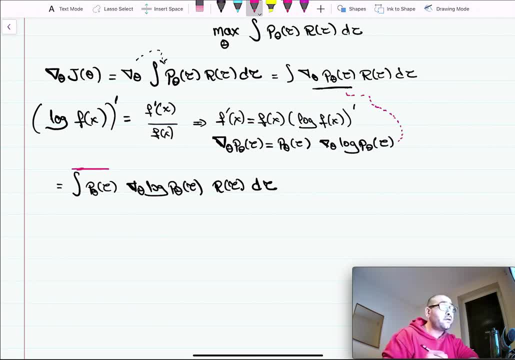 And then you have that chunk there, So you have this chunk here which is kind of your function, right? So so that's kind of your function. Oh for, sorry, without the detail. the detail needs. we need it, right. 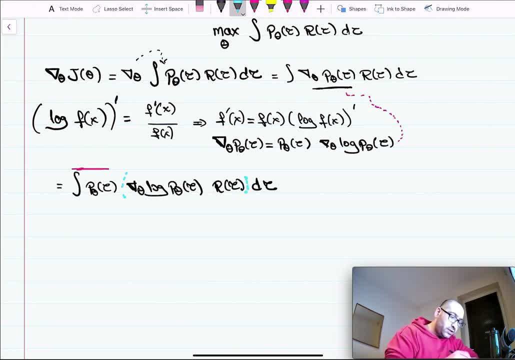 So so times this function. So so what you can already- you know, you know- understand from this equation is that, oh, okay, I can actually write this as expectation under tau Sampled from p: theta Of tau right. 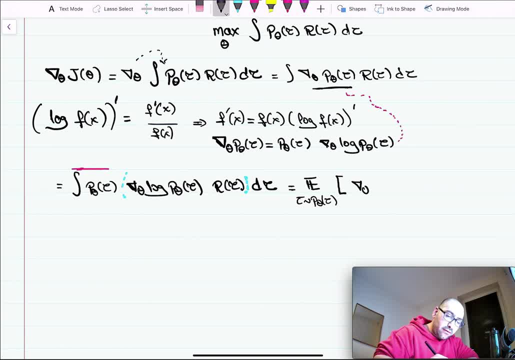 And multiplied by or off, Sorry, the gradient of log of p, theta of tau, Okay, r of tau, Yeah, So. so now we're getting very close to a, to, you know, standard reinforce with. one last thing we need to talk about: 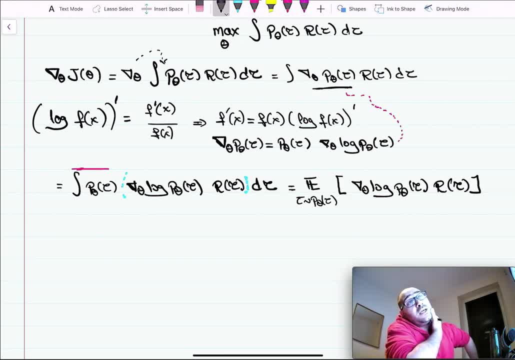 So at this stage you should be a little bit worried, because- because okay, you're, you're- I'm asking you to compute for me the gradient of a log of some probability density, right, And in that probability density there's a chunk which we do not know. 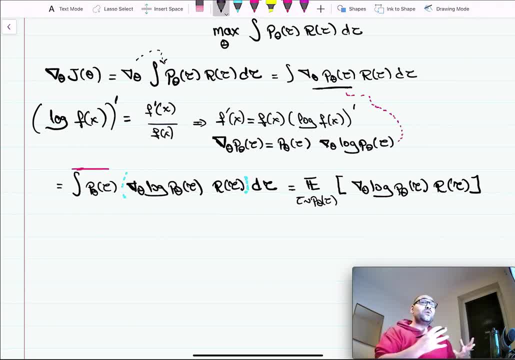 And that chunk relates to the transition model, right? Remember we said: RL assumes we don't know the transition model, right? So so in other words, now if we look at p theta of tau again, right, So let's look at that again. 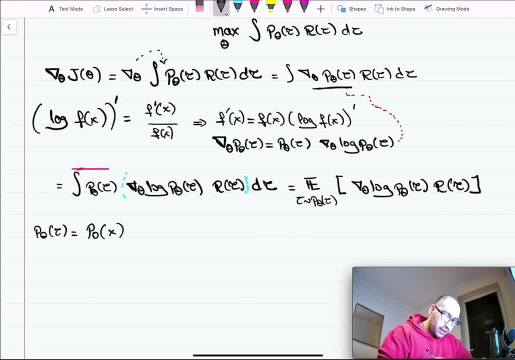 You realize that, as we said, p zero, right X1, then you had this product over time and then you had p of xt plus one given xt ut right And before we had the policy pi of ut given xt agree. 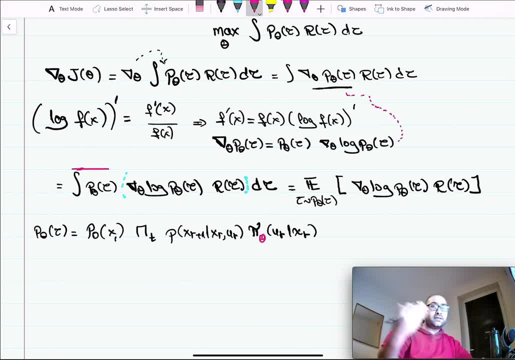 But now remember that we parameterize this by theta, right? So it's kind of that's why we called it p theta. you know of tau. Now you're going to be careful a little bit, right? Because? because here 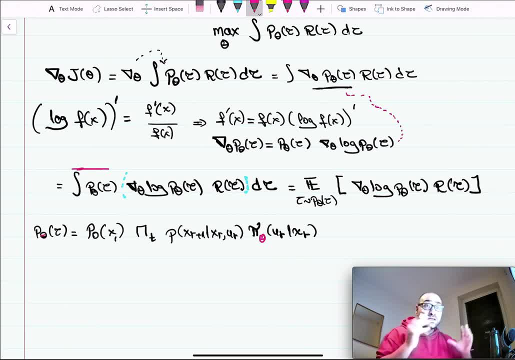 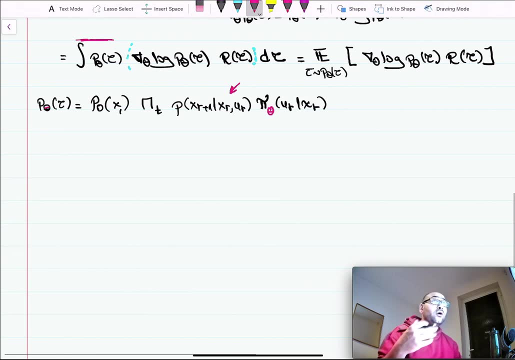 If you are in need to compute p theta of tau, somehow, you need to have knowledge about this transition model here, which we do not necessarily have. So now the question is, or the cool thing is that, what happened is that this log trick we introduced. you know this log trick, we introduced it. 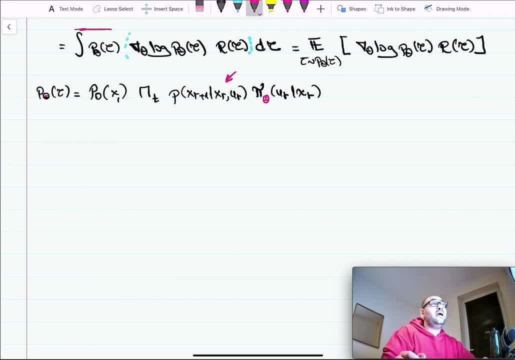 actually enabled us to also get rid of a very messy ingredient, which was this product over these transitions Models, this product over these transition models. Now, why, you might say. I mean, let's check that. So so remember, we need log p of theta in this equation. 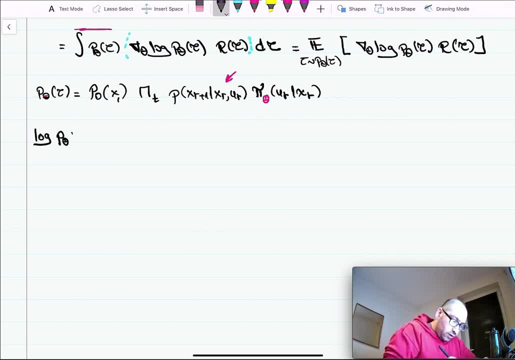 All right, so let's do log p of theta. So log p theta of tau is what? Well, okay, Now this is a product of three terms, right, So it's log of a times b times c, which can be written as log of the sum. 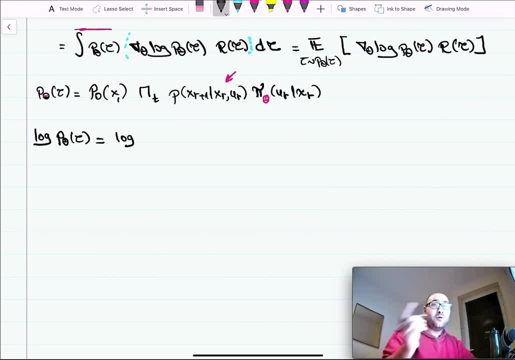 So so you can say, okay, this is sorry, sum of the logs. So so you can say, okay, this is log of p zero. Right, Then you have this summation over t of log, of log of p of xt plus one given xt, ut plus the. 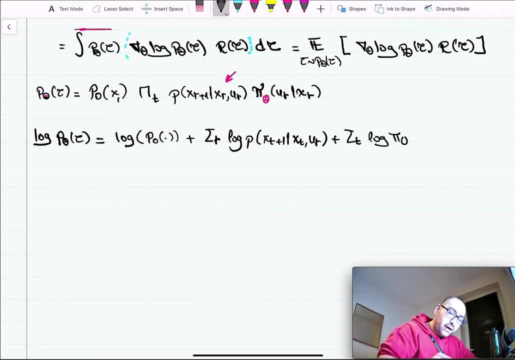 summation of log of the policy right Pi theta of ut given xt right. That's that's what we know Now. it's actually interesting Because we want the gradient of that, We just don't want the log only. 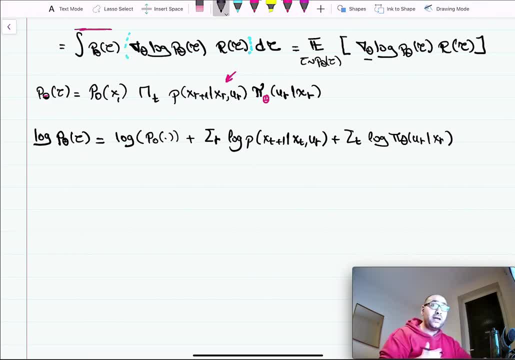 Remember, there's this gradient part here, So we also want the gradient of that. Okay, so now, if we take the gradient with respect to theta of log of p, theta of tau, Now you need the gradient of the first, the log of p zero. 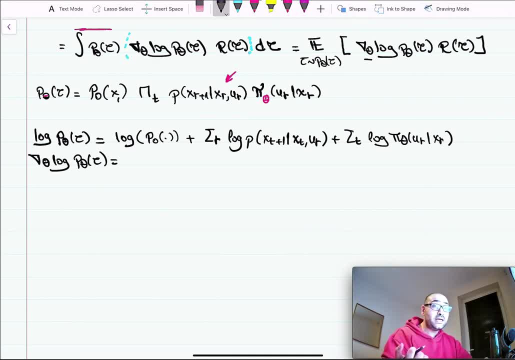 But hey, that zero, because it does not depend on theta. Similarly, this transition model, which was the mess which was hard to deal with, also vanishes, goes away because, you know it does not depend on theta, And the only thing we're left with is the gradient of the policy. 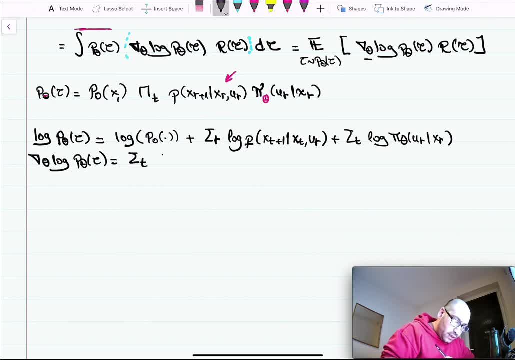 So now we end up with the summation over t of the gradient with respect to theta of log of pi, theta of ut given xt. So what effectively we're able to do now is, if you know the structure of the policy right, So say: this: is this neural network without this Gaussian? 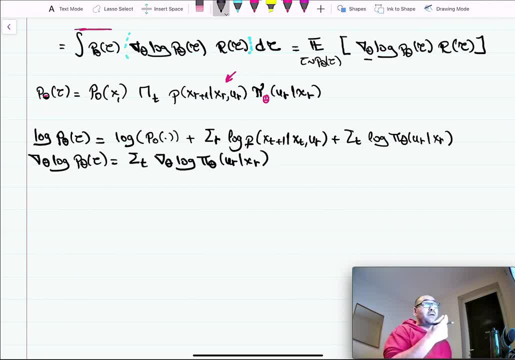 Well, okay, then you just can do autodiff. Okay, you give me a state and an action, Sorry, you give me an action and then I can just autodiff in order to get this gradient. So now, this is pretty cool. 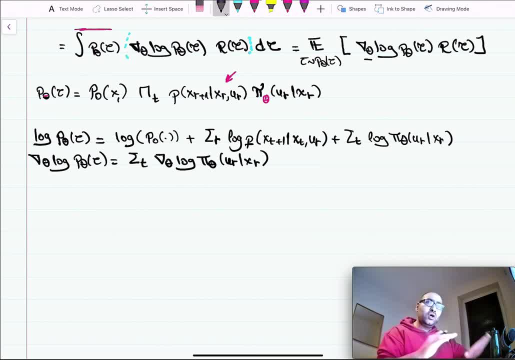 But now you might say: okay, where did these actions come from? and stuff like that. We're going to, we're going to go into that in a second, But now I'm just. what I'm going to do now is I'm going to substitute my derivations. 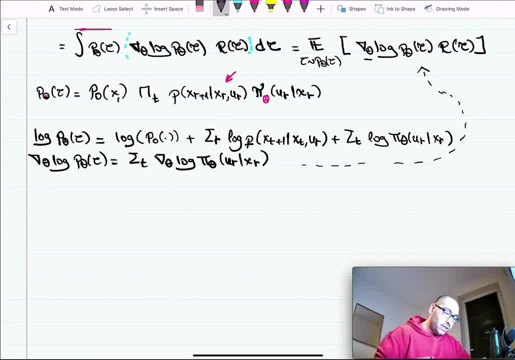 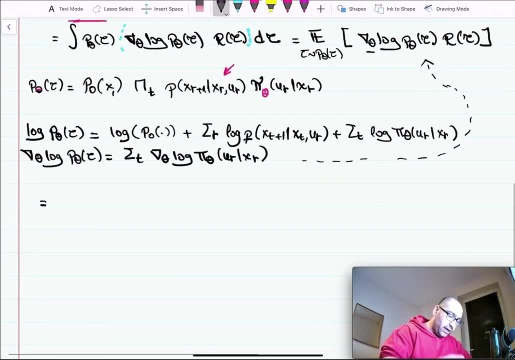 You know what I've just done back in this equation And now I can say that, okay, this, remember this equation- is the gradient of J, right? So I can say now that the gradient of J can actually be written as the expectation over. 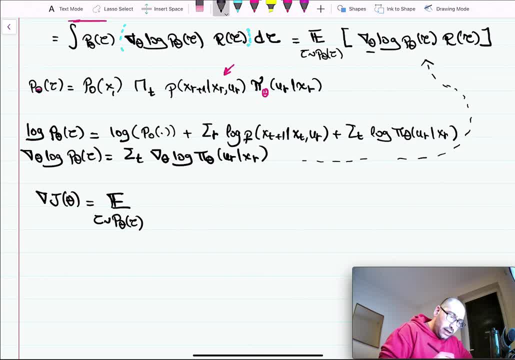 tau of p, theta of tau, And then you would have here the gradient. But now, please remember, instead of gradient log theta, we just have the sum of the gradient, Right, So sorry? So I should write, maybe here the sum, the summation over time of the gradients, of the log of. 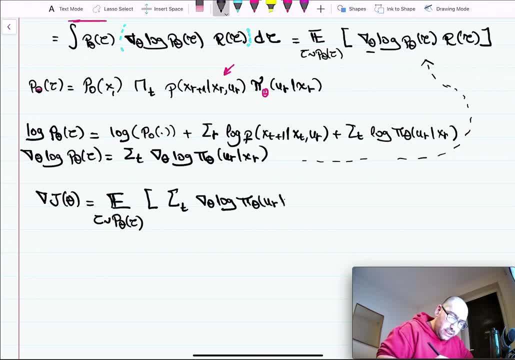 pi theta of ut given xt, And then here you multiply that by r of tau. Okay, all good, So so now we have this equation, That's the gradient for us, And now please notice that this enables you to do Some algorithm right. 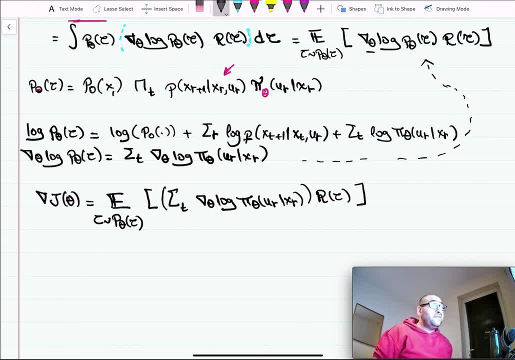 Like this enables you to code something up, because now what you can do is you can do a Monte Carlo estimator of this, of this component of this gradient, and then compute a, you know, a, an estimation of this gradient, And then you do a gradient step in theta right. 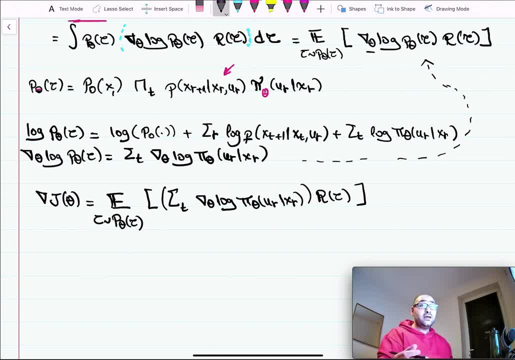 That's. that's, that's a typical algorithm, What you can device now. Now the question is: okay, how would we sample right? I mean in in in ERM map problems, It's easier a bit to sample. 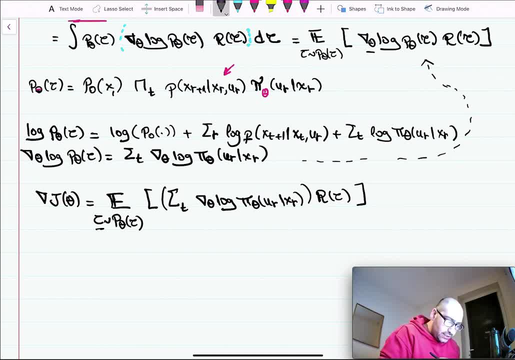 But here, what you need to do is you need to sample a trace tau. right, You need to sample a trace tau by following p? theta of tau. Now, you actually do not need to know p? theta of tau, but you need to be able to sample from it. 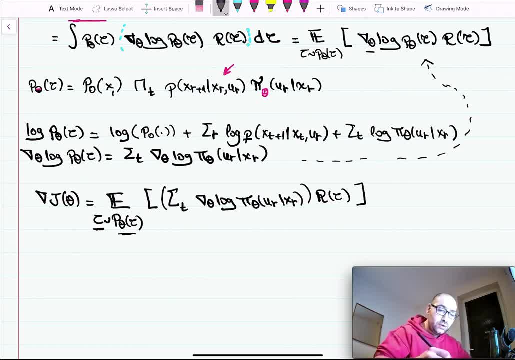 And the way to sample from it is pretty simple, Because what you do is you start at some x0, which which you know you, it comes, sorry, x1.. We call this right. So so you sample something. 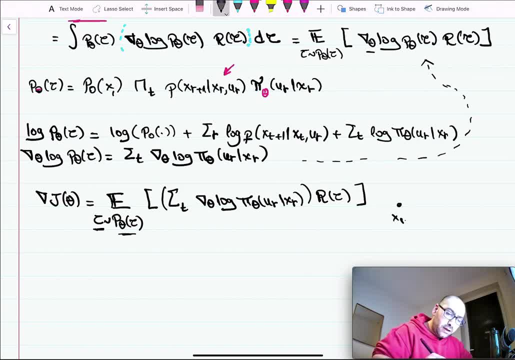 Starting from x1, sampled from this initial state distribution, And then from there you take an action according to the policy pi theta. It gets you to x1 according to p, And then you repeat this up to some horizon t, And then you sample a lot of these right. 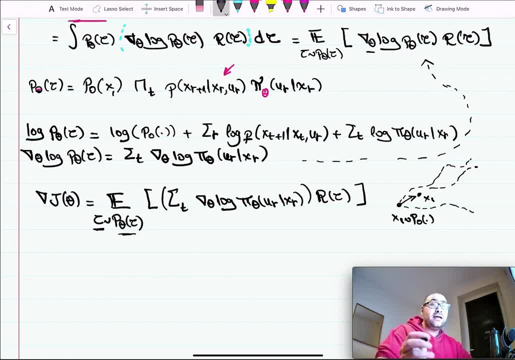 So you sample a lot of these traces, okay, And then you can now estimate this. you can estimate the sorry, this equation, this equation here, Using, you know this equation here, Using these Monte Carlo samples. So you start, you run your simulation. you know, you gather a lot of these traces. 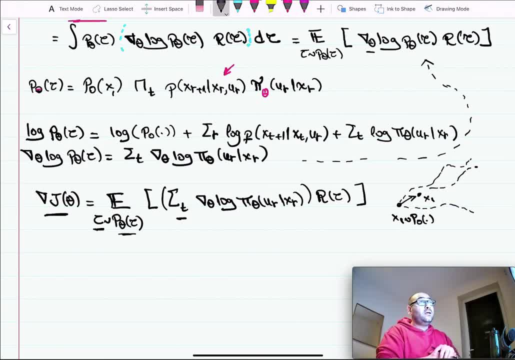 And then you know you can do one step in this update. Now, the problem with this estimator is that it exhibits high variance, But we're not going to dig into that yet. There's another alternative of that, which is like reparameterization of these gradients. 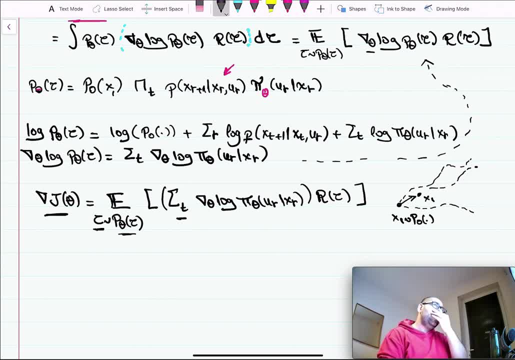 You can. we can also look at that, but we will look at it way later And it turns out that it's not always guaranteed that that will produce for you lower variance than this slightly lower gradients ratio method. you know this simple, simple method. okay, so all right, so so that's. 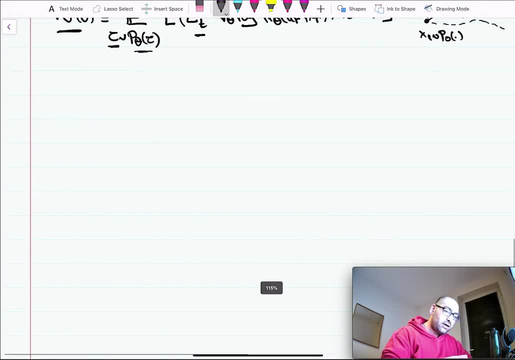 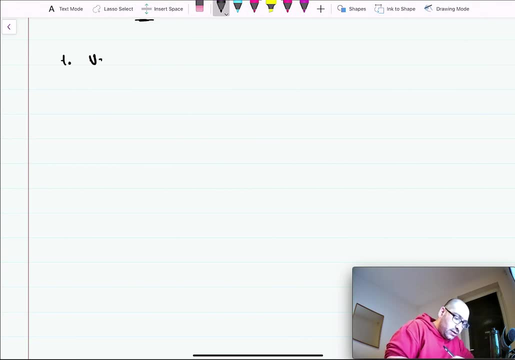 what we have. so now, what would our algorithm look like? okay, so, so this is kind of the policy gradient method now. so what you're gonna do is, in the first step, all right, using using some policy, using PI, all right, yeah, PI, let's call it PI, theta, alright. sample traces from the environment. sample traces from the 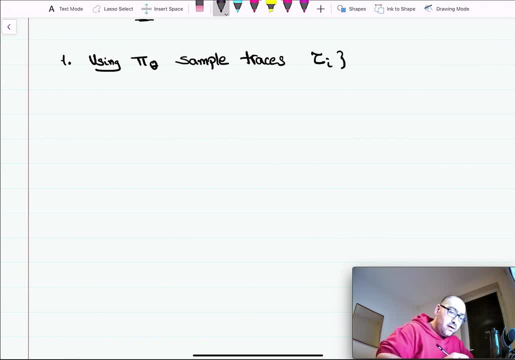 environment. let's say we sample tau. I you know, I don't know we sample n of them. all right, just some kind of them to. we are gonna now update theta, so we're gonna just compute an update of theta so we're gonna say, okay, update theta, update. 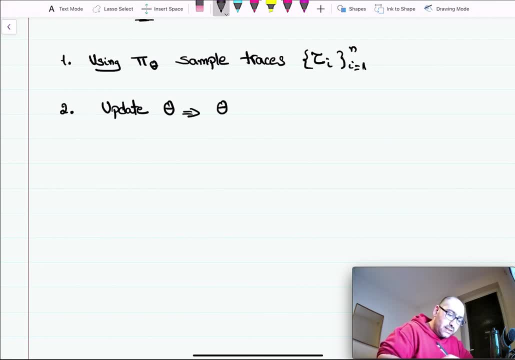 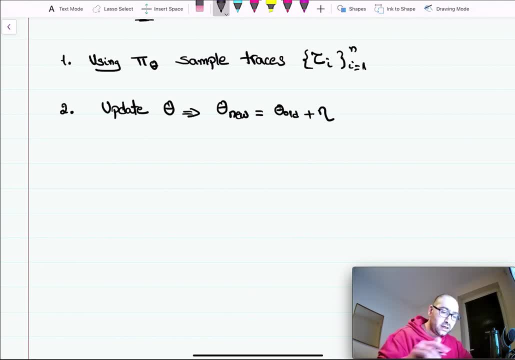 Maybe you decay this learning rate. It's really up to you. I mean, there are some works that decay, There are some other works that don't, and things still work. We do not really understand what's going on here mathematically. 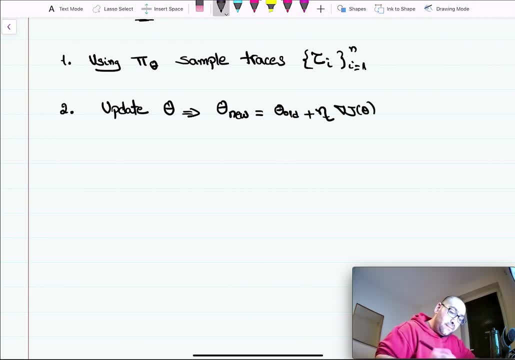 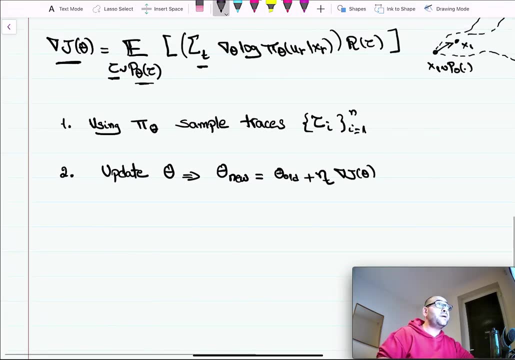 Times, as we said, the gradient of j of theta right And now, since we cannot estimate j of theta exactly, because j of theta has this expectation, as you see in this equation, and we cannot compute this expectation in closed form. 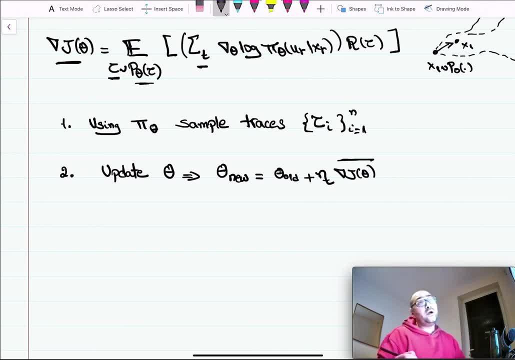 what we're going to do is we're going to write a bar above it, where a bar simply means a Monte Carlo estimator of this equation above right. So this bar simply means we're going to do a Monte Carlo estimator of this equation above. 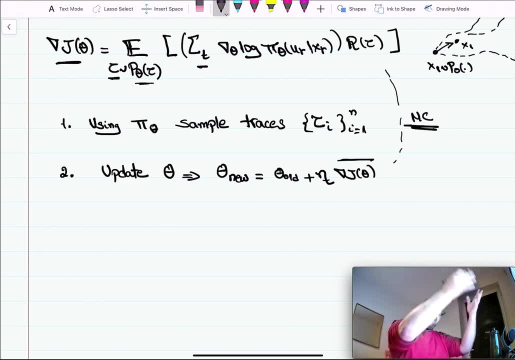 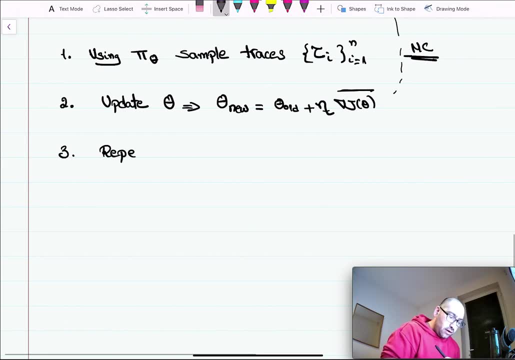 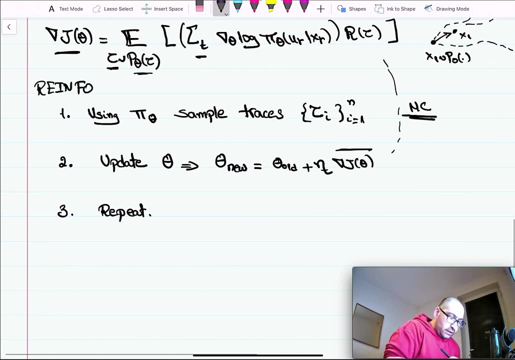 How do you do Monte Carlo? Well, as we said here, you sample traces, then you do an average Of this equation and then three repeat. So that is kind of what the simplest algorithm, called reinforced, looks like. And yeah, and I mean, this is not necessarily a very well-behaving algorithm. 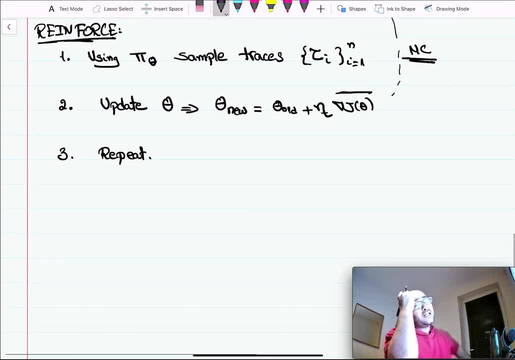 but the reinforced was one of the earliest algorithms, dating back to Williams, I think in 19.. I do not remember the exact date, But it is a pretty old algorithm. and yeah, it just operates in this way: First you sample traces, then you update the policy, using like a stochastic gradient. 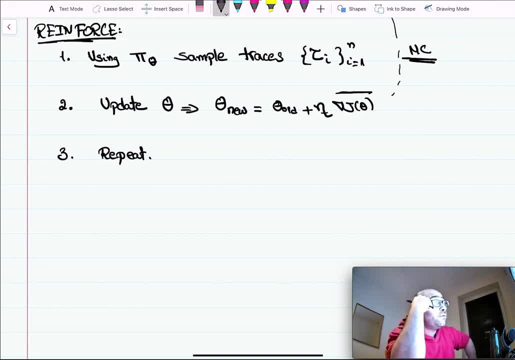 by doing a Monte Carlo estimator, using the log trick which is derived, And then we repeat this process over and over again. Now the big problems in reinforcement learning start happening, because to estimate this gradients, here you know, you have variance introduced. and now this variance 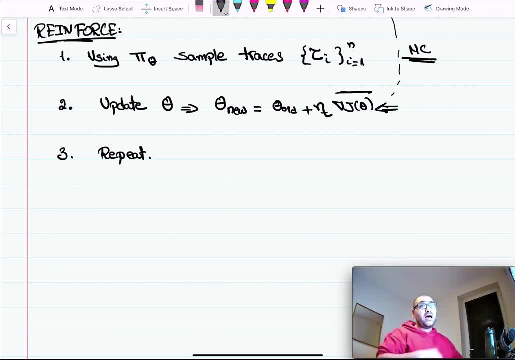 it can affect your conversion speed. So you know, the higher the variance, the worse your conversion speed is. And then there has been some tricks to do, which we will talk about next time, For example, subtracting a baseline actor critic method. you know stuff like that. 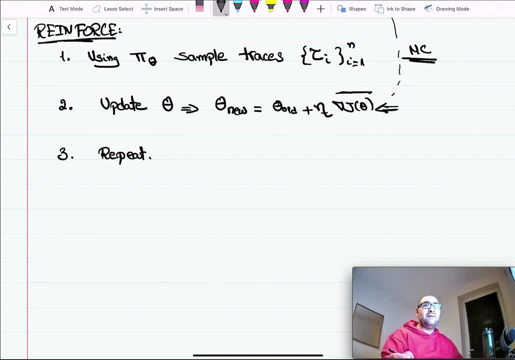 They all are really doing the same thing, which is described, But now they're trying to, you know, somehow kind of reduce the variance and have a better form of an update than the update we did here And now. to actually implement this also is very simple. I mean, like if you go to OpenAI Gym, you will see the interface that allows you to, you know, interact with the environment, and then you will just take an actions and then it will return for you some state and reward. 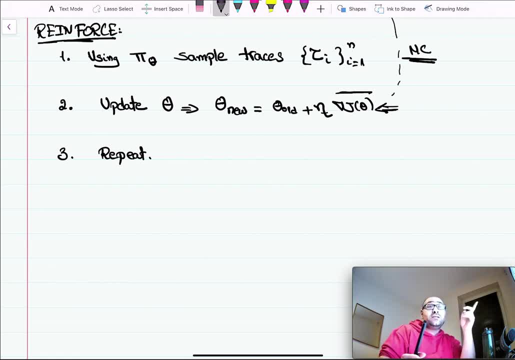 And then, based on that, you can just do this estimation and then yeah, and then we're good to go. So, believe me, I am not good at coding, but I actually have coded this method myself multiple times And, yeah, in simple systems like CardPool and stuff like that, it works really well. In harder systems not so much, And that's why we needed all the new stuff like TRPO, PPO and stuff like that. 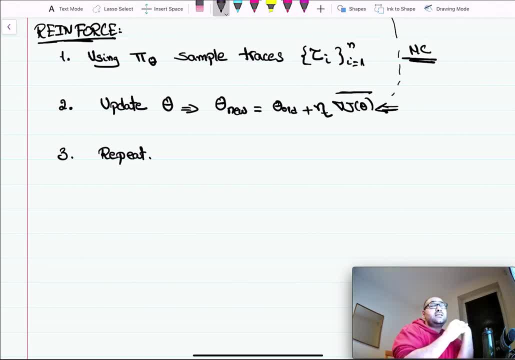 So next time we're going to continue discussing these things, I think maybe next time I will talk a bit more about the baselines and, you know, various reduction kind of techniques and maybe touch a bit on re-parameterized gradients before jumping to discrete the states, discrete actions, sorry. 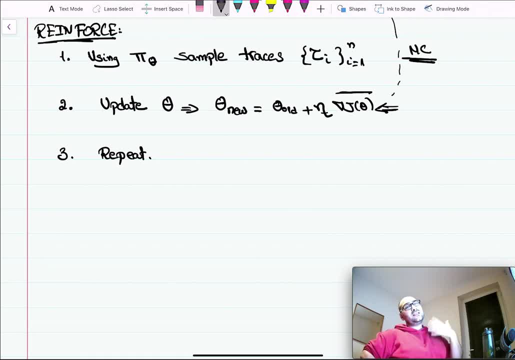 So, as you see here I described the continuous action setting and the discrete action setting. you still would be able to do policy gradients, because you can now parameterize the policy in such a way that the neural network outputs discrete actions And yeah, and then we can go from there. 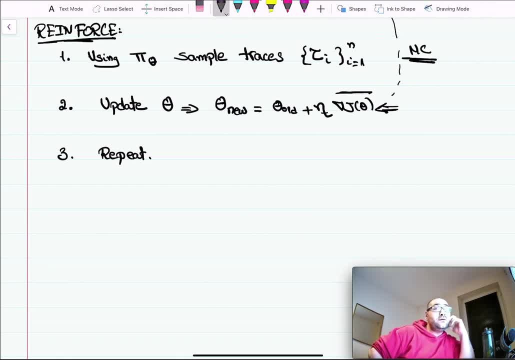 So, yeah, so thanks for listening And yeah, I'll see you next time, Hopefully not far away. It all depends on how busy things get. Yeah, Thank you, Bye, bye.